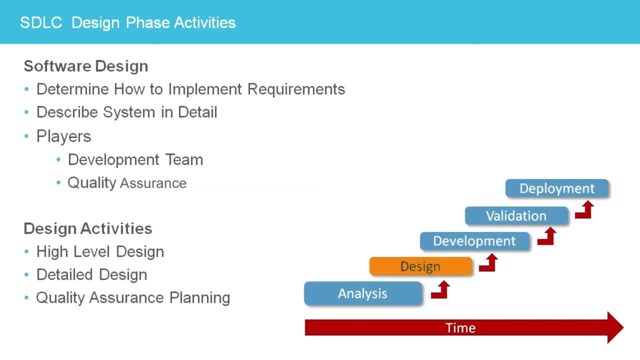 for their detailed design. During detailed design, large modules will be broken down into smaller ones with their own descriptions, interfaces and diagrams which show how to implement the module and software. Design engineers often use prototyping, investigating areas that are unclear or unknown to gain clarity and determine a design approach. 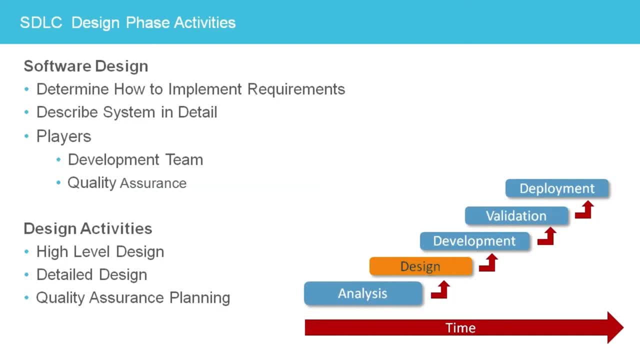 Stakeholders and customers review and comment on GUI wireframes and screen layouts that show the flow through the product's user interface, And database designers add additional detail to the logical entity relationship model to create the final database schema. Quality assurance is also hard at work. using the requirements to develop the strategy, the 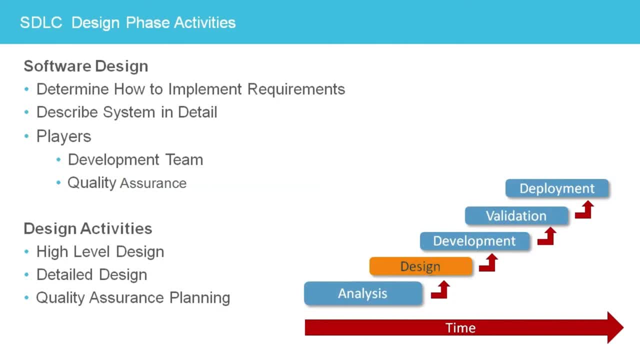 QA team will use to validate the final system. Areas of QA planning will include how deep defects will be reported and tracked, how software will be delivered from development to the QA team for validation and how the different tests will be performed. Planning also includes specifications for the isolated test environments, An area of special interest. 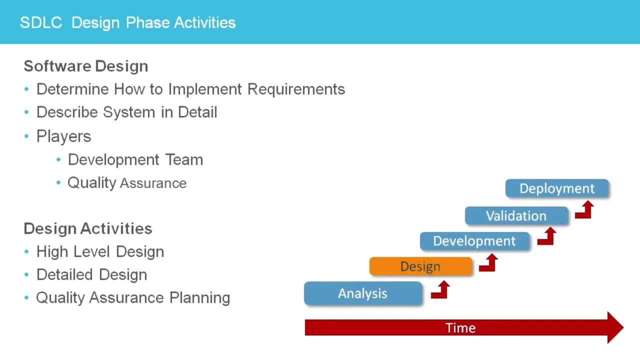 is how acceptance testing with the customer will be accomplished, as this determines if the customer will accept the implemented system. During this phase, build out of the development environments must be completed, as they will be needed to implement the application in the development phase that comes next. 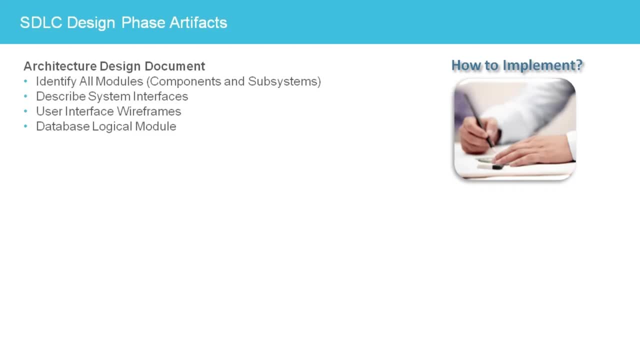 The design phase activities result in artifacts that are used in the development phase to implement the final system. The architecture or high-level design document gives a blueprint of the entire system which will be built. It will include the software architecture which specifies. 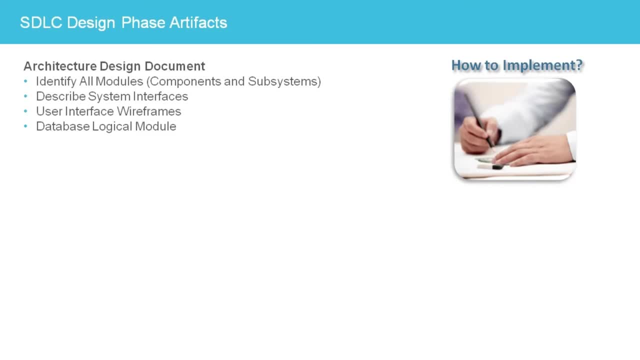 the modules and the interfaces between them and external systems, as well as communication methods. The user interface flow will be described with the wireframe screens, and the logical database model will also be included, showing entities and their relationships. The architecture document will include many diagrams, such as UML system diagrams and 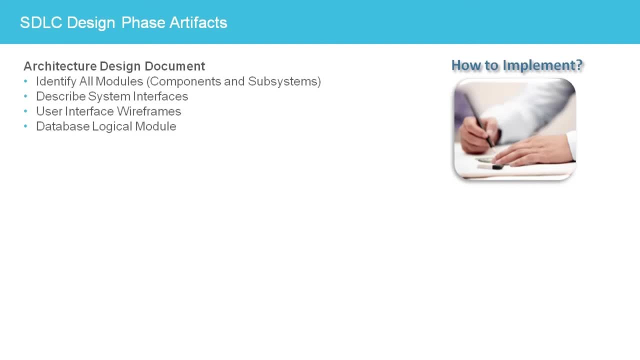 database entity relationship diagrams. However, it will still primarily specify what should be implemented, without details of how to implement it. The details of how to implement each module are specified in the detailed design document For each module. the detailed design document describes the algorithms and data structures. 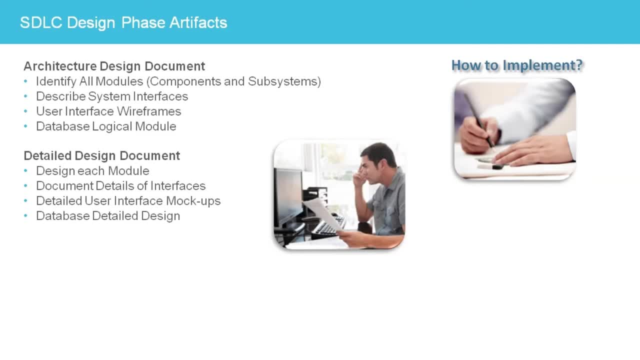 used detailed design diagrams and detailed interfaces. The interfaces will include the exact data items transferred between modules, along with their datatypes and their properties, type and other attributes like permanence and scope. Detailed design diagrams may include UML diagrams that show the structure and behavior. 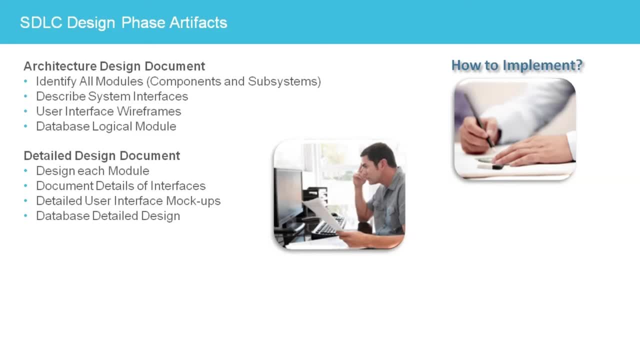 of objects in the module: data flow diagrams, flow charts and sequence diagrams. Some projects will use pseudocode to define the actual structure of the code which will be implemented for each module. The user interface will be mocked up to demonstrate the look and feel of the final screens. 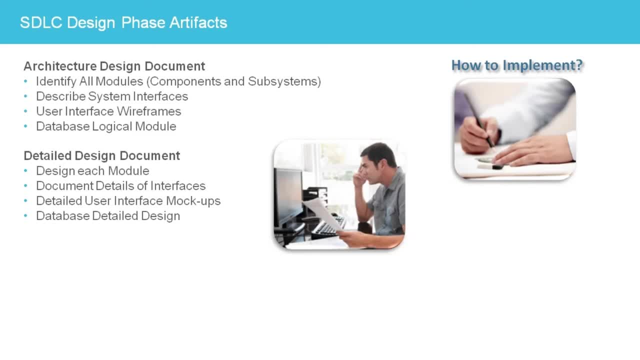 the user will experience And the database detailed design will be created which specifies the details of each table, including column names and data types, as well as column and table constraints. Views, triggers, stored procedures and other database objects will also be specified in detail. 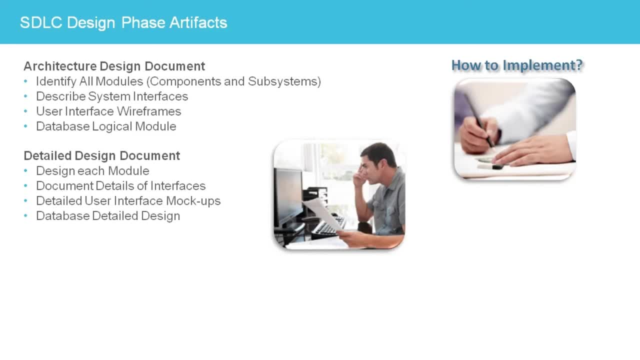 as well as the method of how users will be authenticated and what database objects will be authorized for the different roles. The resulting detailed database design will be used to write the database schema In distributed systems. the data dictionary will also be created to specify the meaning origin usage. 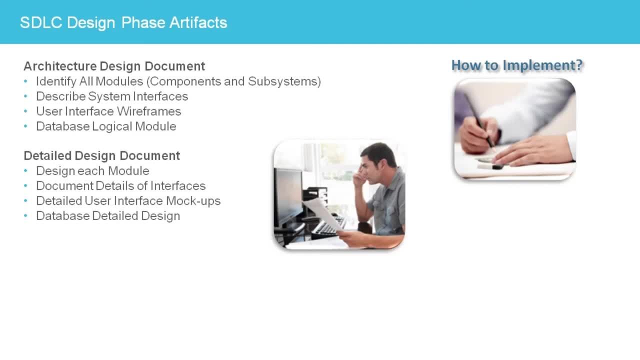 and format of each data item and the relationships between it and other data items in the production environment. All the planning done by the QA team is captured in the quality assurance plan document. The quality assurance plan describes the data structure, the framework and the details of the system. 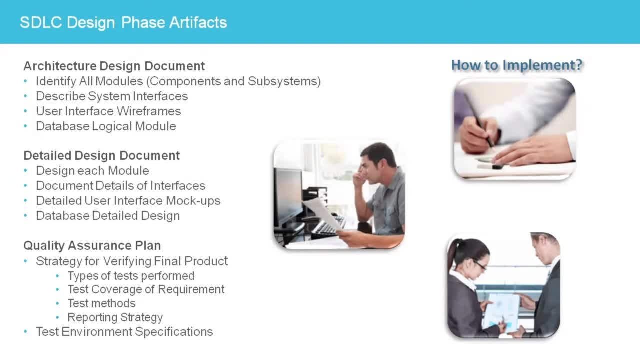 The quality assurance plan describes how the validation strategy will be implemented to verify the system and ensure it is of high quality. The quality assurance plan will include a schedule of the QA activities throughout the project and the documents that will be produced in each project phase.